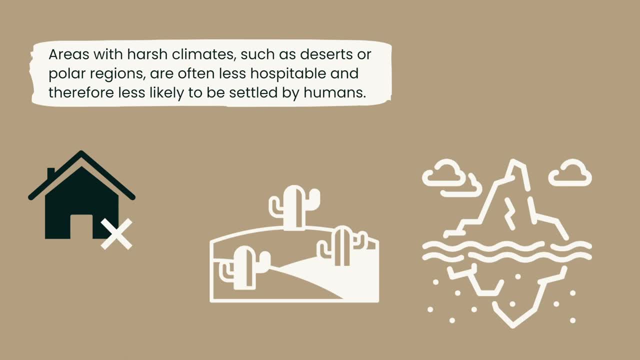 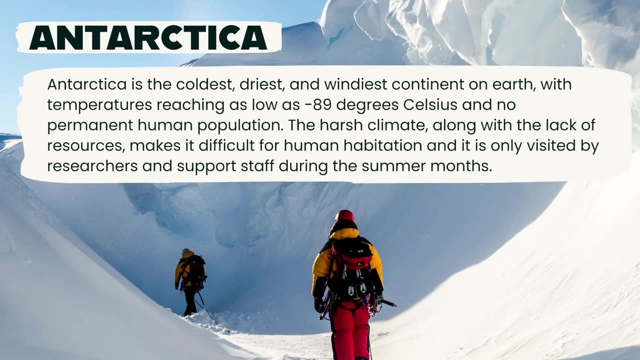 by humans. The environment can also influence the type of settlement that is built, such as whether it's a city, a suburb or a rural area. One extreme example of this is Antarctica. Antarctica is the coldest, driest and windiest continent on Earth. 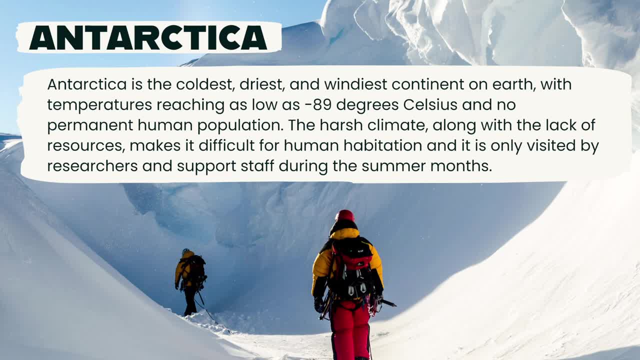 With temperatures reaching as low as negative 89 degrees celsius and no permanent human population. The harsh climate, along with the lack of resources, makes it difficult for human habitation, and it's only visited by researchers and support staff during the summer months. 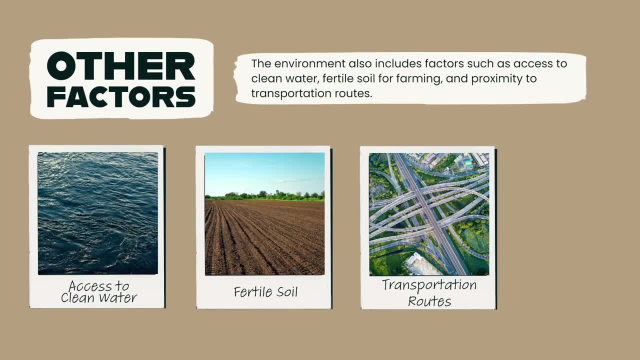 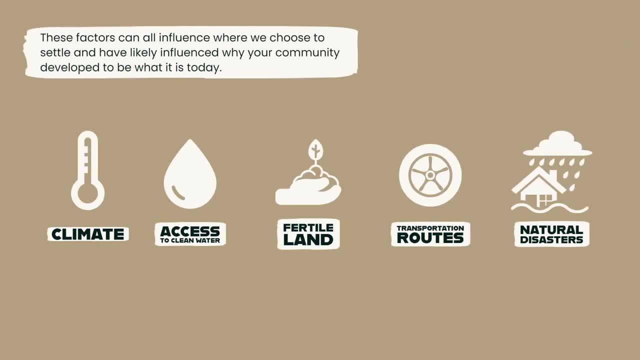 But the environment isn't just about temperature and natural resources. It also includes factors such as access to clean water, fertile soil for farming and proximity to transportation routes. These factors can all influence where we choose to settle and have likely influenced why you might want to move to Antarctica. 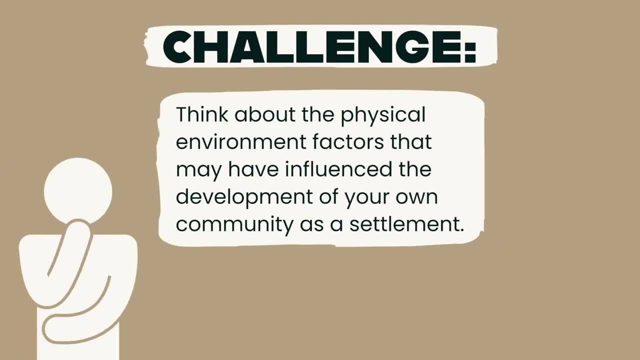 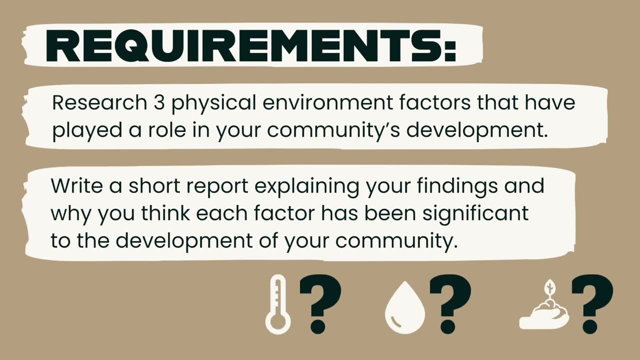 So here's a challenge for you: Think about the physical environmental factors that have influenced the development of your community as a settlement. Your task is to think about your own community and research three physical environmental factors that have played a role in how it's been. 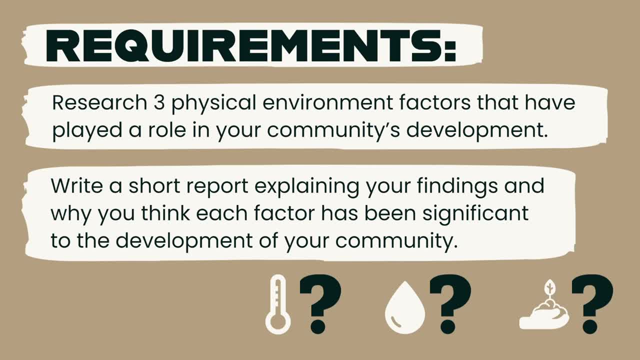 developed. These factors can include things like the climate, topography, natural resources, bodies of water and more. Once you've gathered the information, explain your findings and why you think each factor has been significant to the development of your community. Write a short. 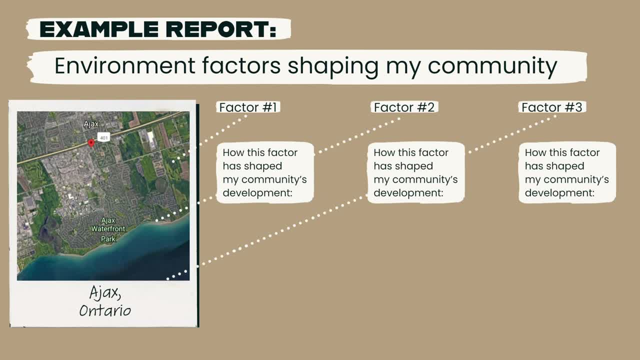 report on the development of your community and share it with your friends and family. You can also create a slideshow explaining all of this information. You may wish to search for your community on Google Earth so that you can see the surrounding landscape and make predictions. 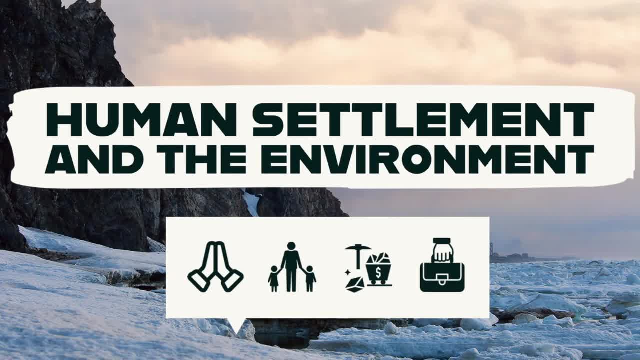 about any factors that may have shaped human settlement there. Be prepared to share your report with the class and discuss the results. Good luck.